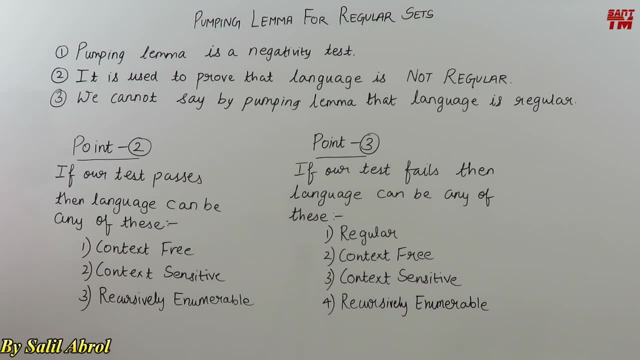 hierarchy, there were four types of grammars: Regular grammars, context free grammars, context sensitive grammars and unrestricted grammars, which each of them corresponded to the languages. The unrestricted grammars corresponded to recursively enumerable languages. The context sensitive grammar corresponded to context sensitive language. The context free grammar. 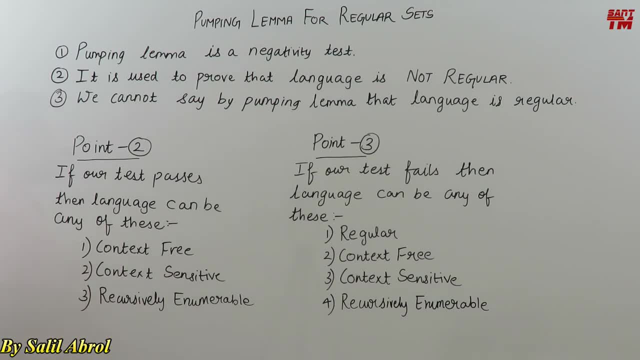 corresponded to context free language and the regular grammars corresponded to regular languages. So the pumping lemma is used to prove that the language is not regular. Then if our pumping lemma- the test to prove that the language is not regular- is passed, That means if we have 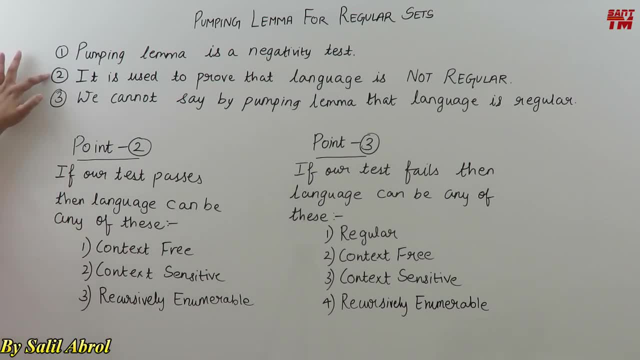 pumping lemma test. that means the point 2 is true. now, if the point 2 is true, then the language can be anyone out of these three categories, because we have proved that the language is not regular. if it is not regular, then it can be either context free it can be, either context sensitive it can be, either. 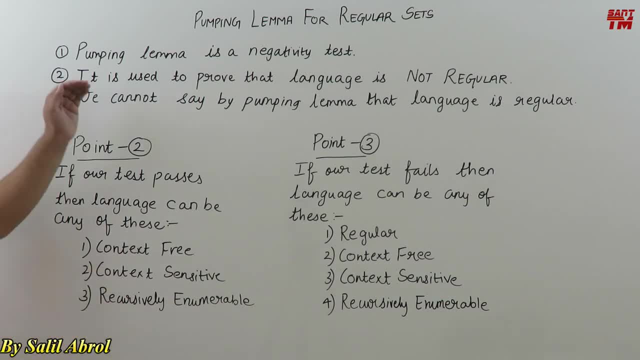 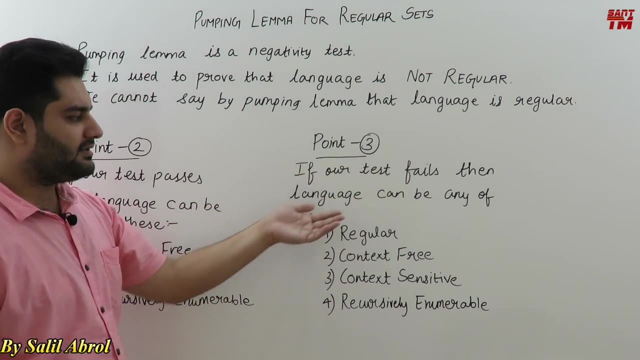 recursively enumerable language. but if our test has failed, we have not passed the test, then we cannot say that the pumping lemma by the pumping lemma that the language is regular. but this is third point- mean if our test fails, then the language can be any of these either: regular language context, free context. 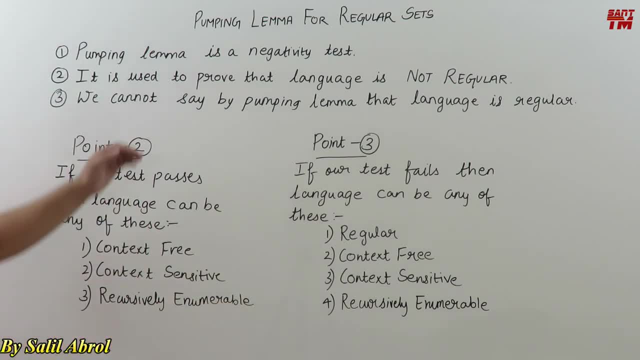 sensitive or recursively enumerable. note this difference: if our test has passed, then the language can be either context free, context sensitive or recursively enumerable. but if our test has failed, then we say it can be any one language out of these three. that means we are only able to. 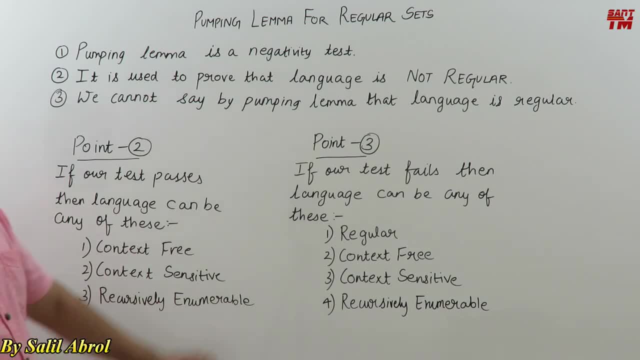 prove that the language is not regular. but we are not able to prove that the language is regular. in the failing part of the test we say that it can be anyone out of the four categories. this is the pumping lemma. so let's discuss about the procedure: how to prove a language to be not regular using pumping lemma. so before 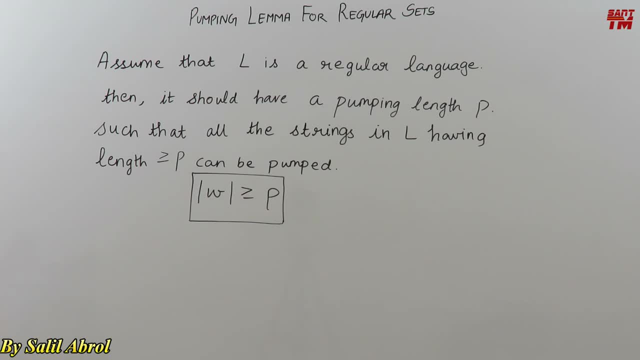 going on to the actual procedure about how to test the non regularity of a language by pumping lemma, consider one point first. the point is we have to assume that the language L is a regular language. any language that we want to test for non regularity by pumping lemma, we will first assume that that language 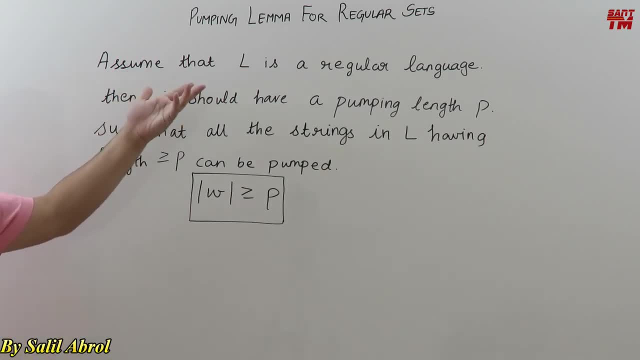 is a regular language. that means first we have assumed that it is a regular language and after, after following the procedure of pumping lemma, we will say that we have contradicted our assumption and thus the languages not regular. this will be the procedure. so assume that L is a regular language. 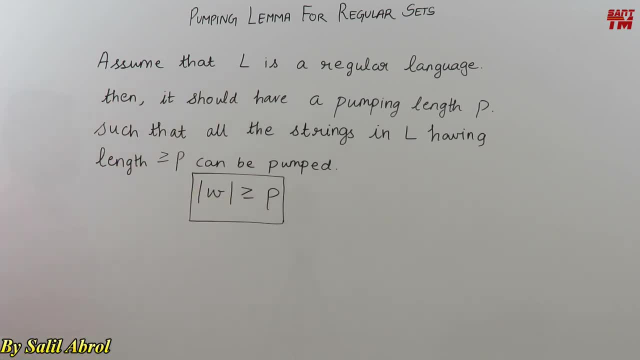 then it should have a pumping length P. what is this pumping length? I will tell you. first consider this point: it should have a pumping length P, such that all the strings in the language L having length greater than or equal to that pumping length can be pumped. so what is the meaning of pumping length and the word? 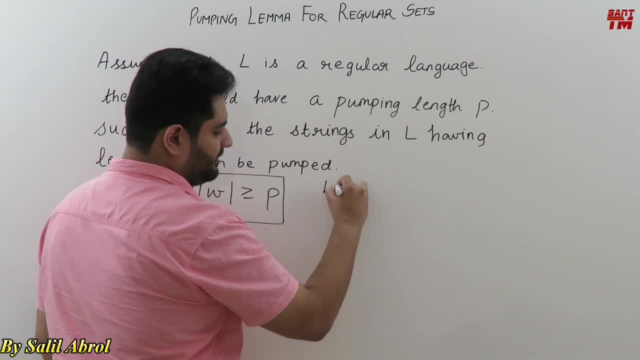 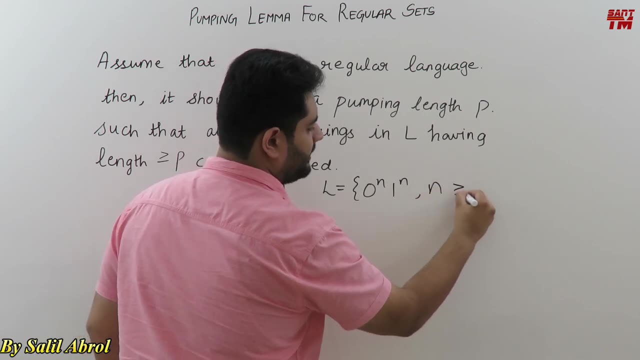 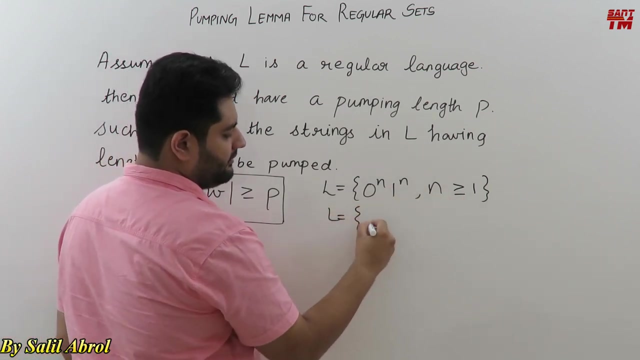 pumped. let's consider it now. suppose L is a language of type 0, n, 1, n, such that n should be greater than or equal to 1, then this language can have strings like: if n is equal to 1, it will have string 0, 1. 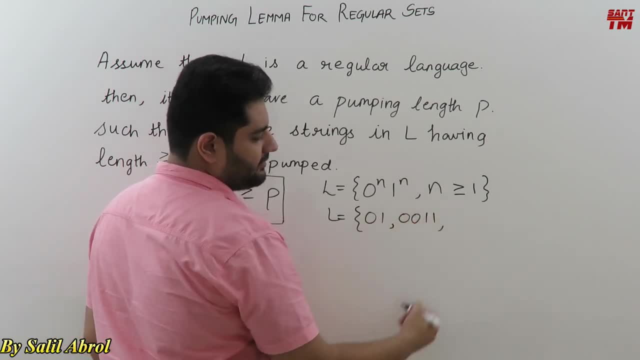 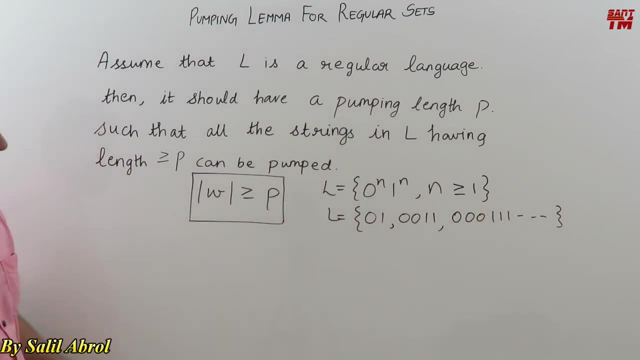 if n is equals to 2, it will have 0, 0, 1, 1. if n is equals to 3, it will have string 0, 0, 0, 1, 1, 1, and so on. it may carry forward. so these are the strings in this language L now. 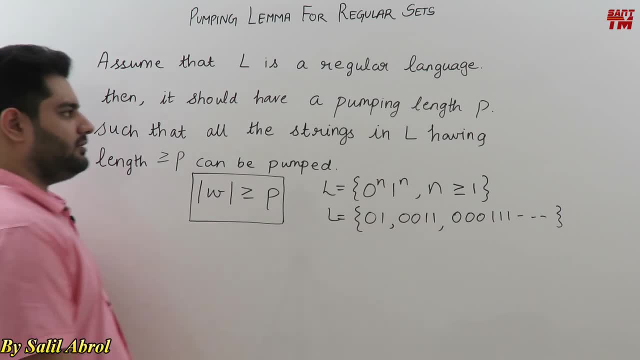 it is saying it should have a pumping length P. now let us decide P is equals to 4. this will also be assumption. we have assumed the pumping length to be 4. this is also our assumption, only. so if P is equals to 4, then the point is saying: 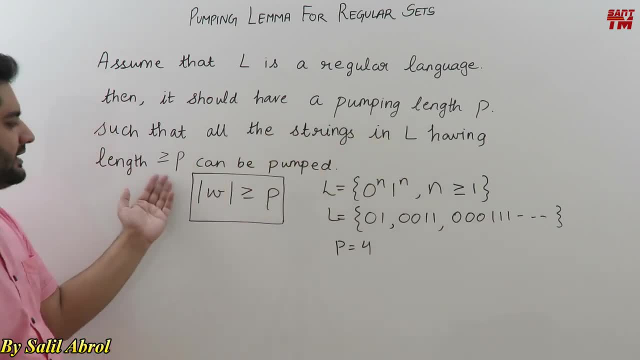 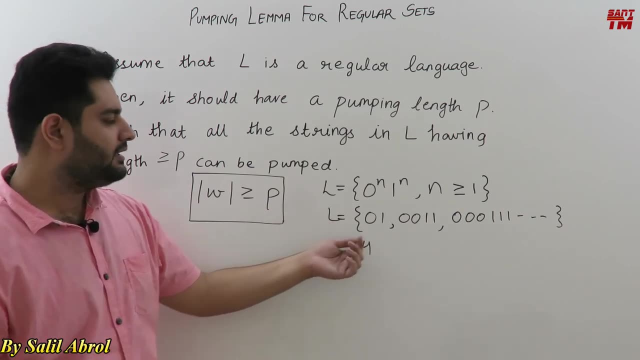 that all the strings in L having length greater than or equal to P. what are the strings in this language that are having length greater than or equal to P? that is, for these strings, this string, all the strings after this string will have the length greater than. 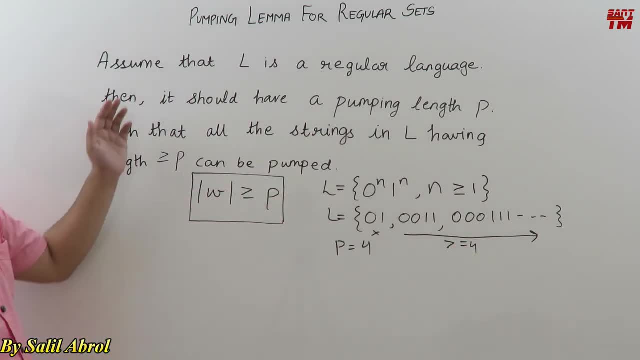 or equal to 4.. So, according to our assumption, if L is a regular language and it is having a pumping length equal to 4, then all the strings in this language having length greater than or equal to 4 can be pumped. That means: 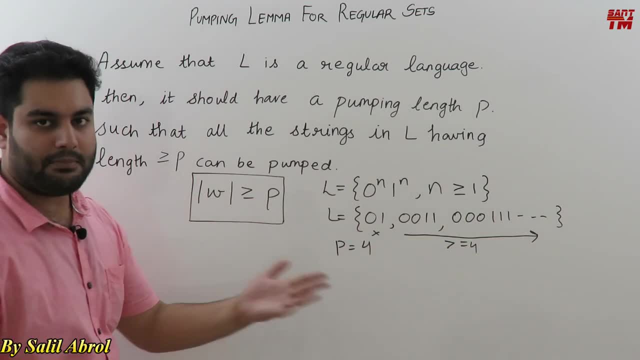 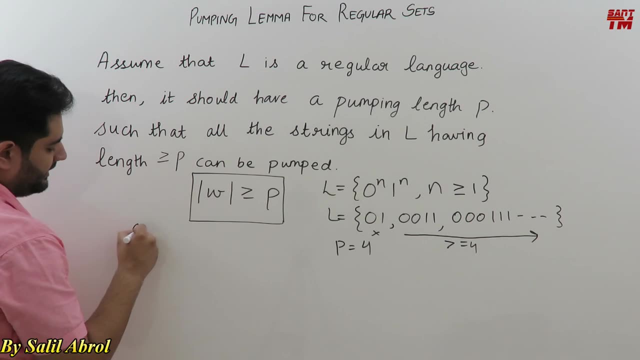 leaving this string, all the further strings can be pumped. Now, what is the meaning of the word pumped? Consider this: If I take the string 0011, it can be pumped because its length is equal to 4.. Condition is greater than or equal to. 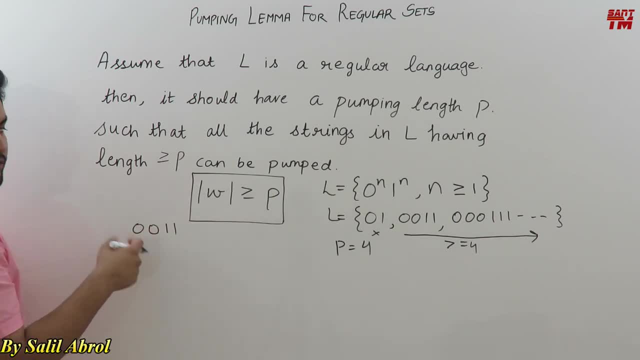 So it is equal to 4.. It can be pumped. Now how to pump a string? See it very carefully. Divide the string into three parts. Suppose this 0 is X, this 0 is Y and these two ones fall in the part of Z. We have divided the string into three. 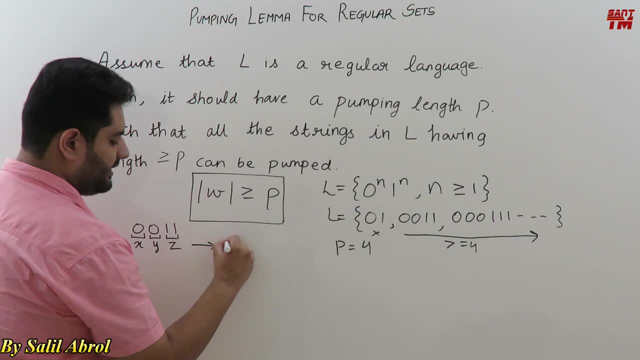 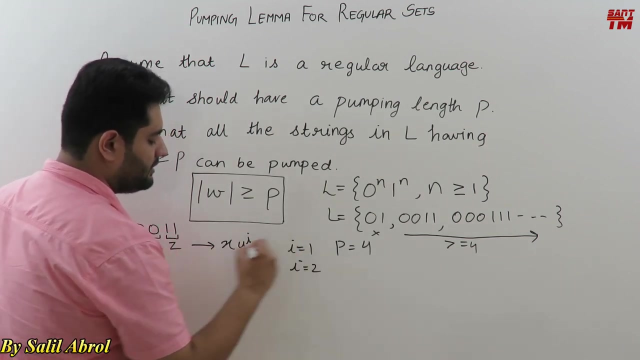 parts. Now consider X, Y, Z. as X, Y, I, Z, Y raised to the power I, Z, such that here I is equals to 1.. Now if I increase the value of I by 1,, if I make I is equals to 2, it. 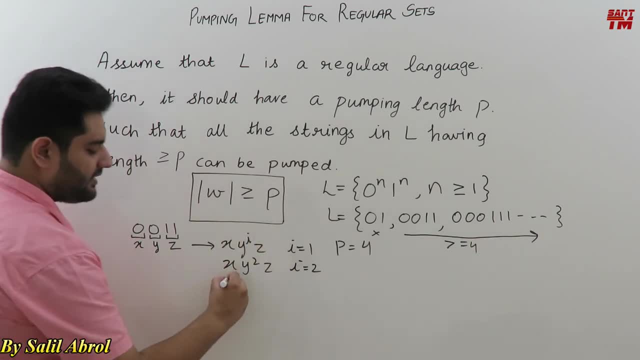 will be X, Y square Z, or we can write it as X, Y, Y, Z. Then the string will be: X is 10, Y is also 10.. Again, Y will be 10 and Z are 2 ones. So after pumping, the string is 00011.. 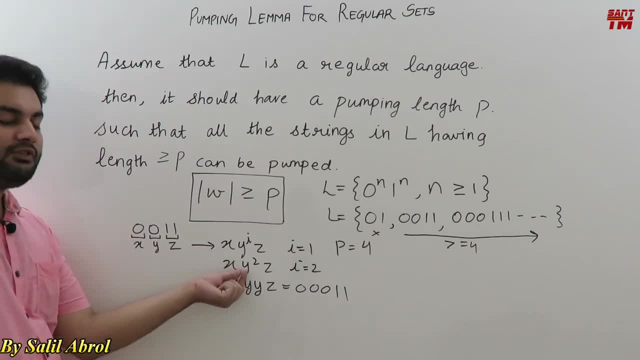 This is how we pump a string. We will increase, we will loop the value of the middle part of the string, that is the Y. We will not even touch X and Z. We will only touch the middle part of the string, that is Y, and loop it continuously. If I 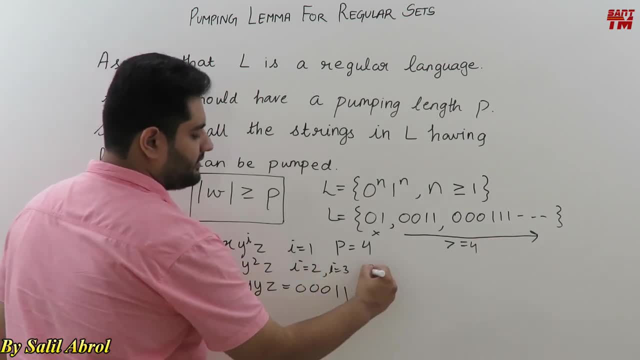 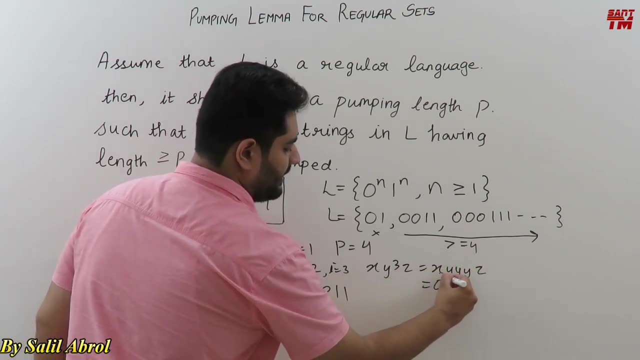 put: I is equals to 3,, then it will become XY3.. z or x, y, y, y, z. It will become x is 0,. y is also 0, 0, 0 and z is 2 ones. So this is how we. 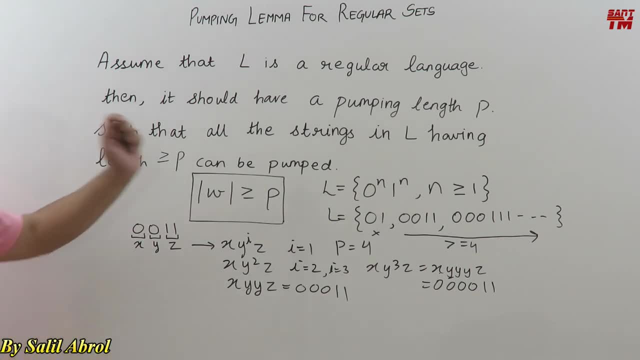 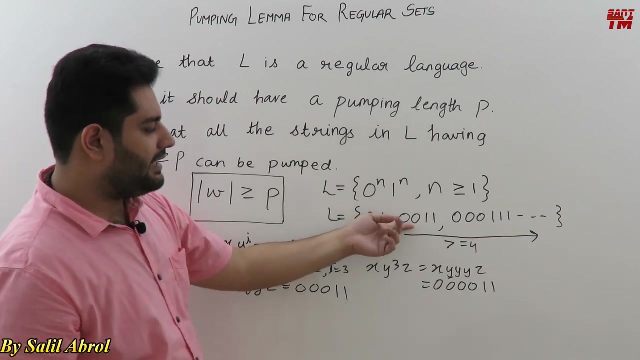 will pump the string. So our assumption is saying that L is a regular language and it should have a pumping length that we have decided to be equal to 4, such that all the strings in L having length greater than equal to 4.. What are all the strings in L, In language L, having greater than equal to? 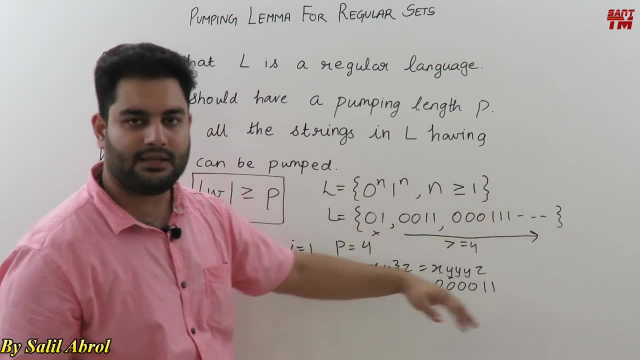 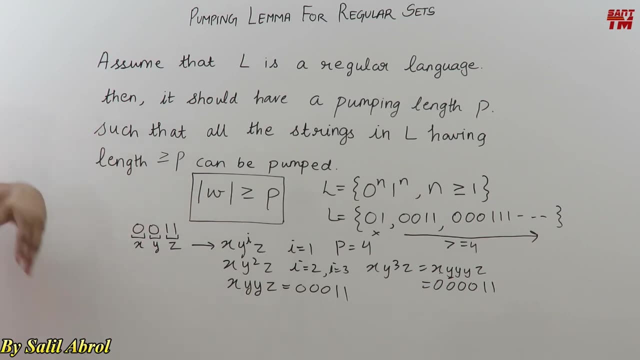 4 pumping length. these are all the strings. These all strings can be pumped. So when we will follow the procedure of pumping lemma, we will prove this whole assumption to be wrong and then say that our language is not regular. We will prove that there is no pumping length P and if there is some pumping 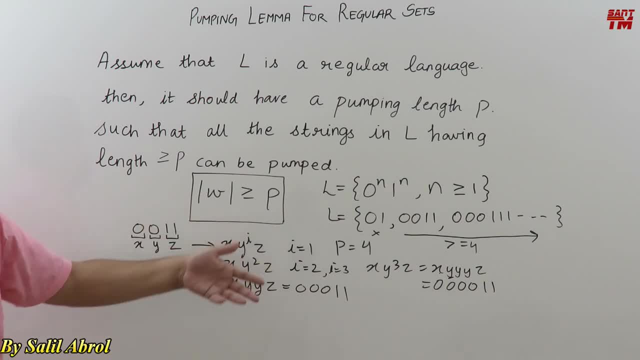 length P, then the string is not be able to be pumped. So we will prove that there is no pumping length P. So it is not following our assumption and thus the language is not regular. So I am very excited to tell you the procedure and then test some examples. Come on, let's begin it. So these 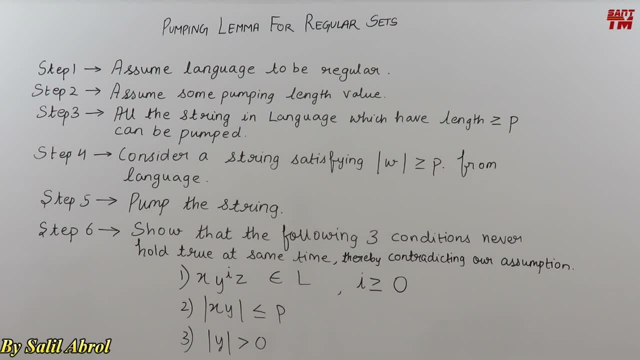 six steps include the whole procedure of testing the non-regularity of a language by pumping lemma. Step number one is: note all the steps serial wise in your notebook. Step one is: assume that the language is regular. Then step two: assume some pumping length value. This was the point that I 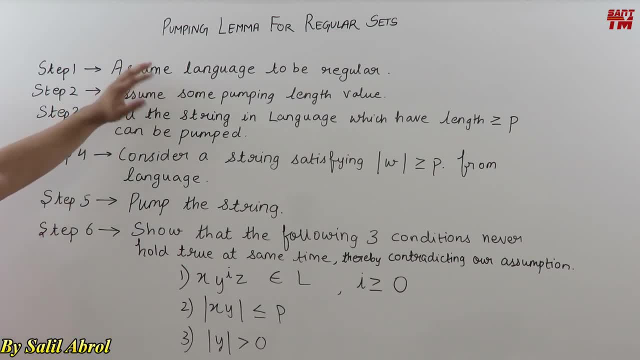 have discussed right now that we have to assume the language to be regular and then we will decide some pumping length And then, in the step three, all the string in the language which have the length greater than or equal to that pumping length P that we have decided in step number two. 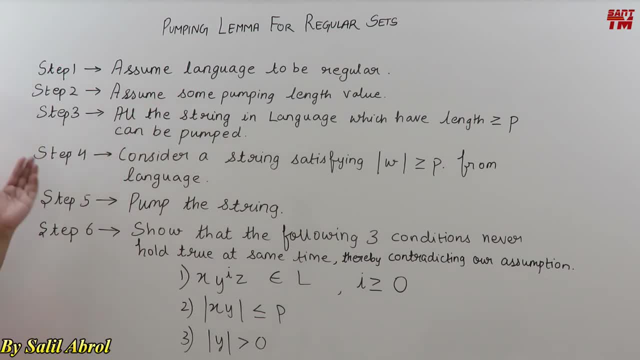 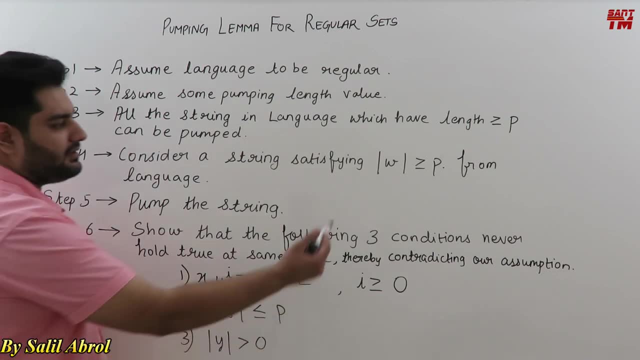 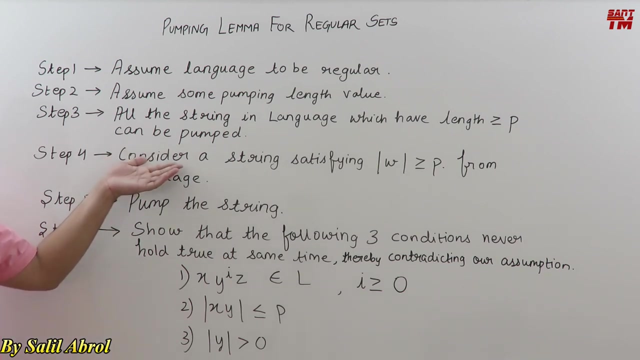 can be pumped. We saw these three points previously. Now step four is: consider a string Satisfying these three conditions. The condition is the length of the string should be greater than or equal to the pumping length. We have to find out any string from the language that we are. 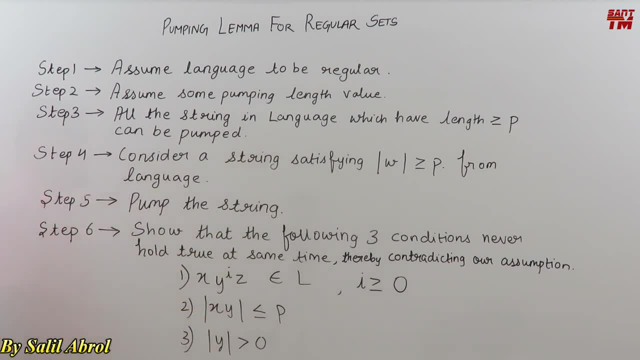 considering Find out that string that is having length greater than or equal to pumping length from the language. Step five is we have to pump that string. I told you how to pump the string. Then, after pumping, consider step number six. Step number six says that show that the following three: 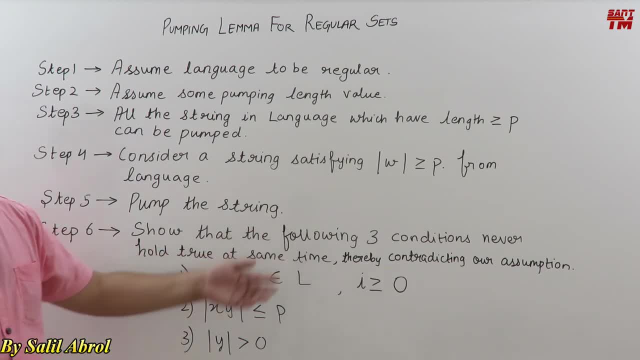 conditions never hold the length of the string. So we have to consider a string, So we have to show that it holds all the length of the string. So now let's consider a string. If we compare the three conditions one by one, Then we see that these three conditions are true at the same time. 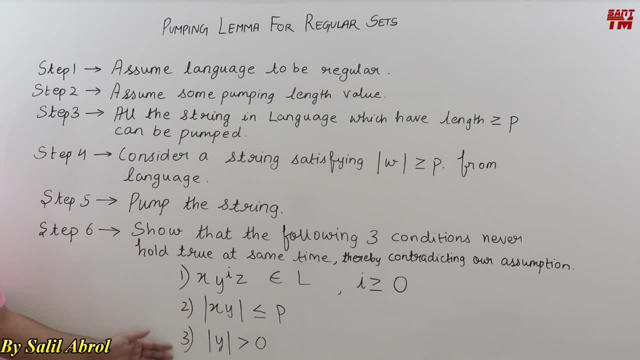 That means sometimes condition number one is false, Other two are true. Condition number two is false and other two are true. Condition number three is false and one and two are true. So we have to show that these three conditions are never true, at the same time thereby contradicting our 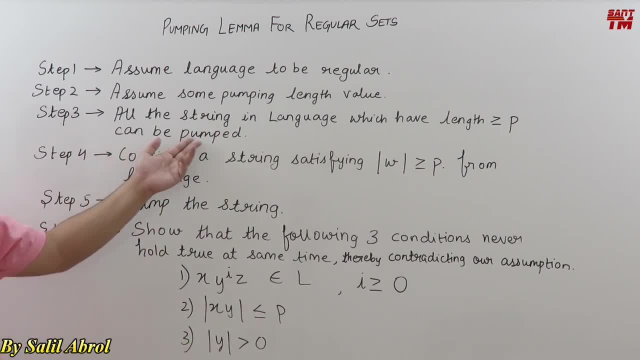 assumption that the language is regular and it is having some pumping length, or there are some strings in that language that has the length greater than or equal to the pumping length. So now let's consider a string. the pumping length can be pumped. it is contradicting our assumptions. these three: